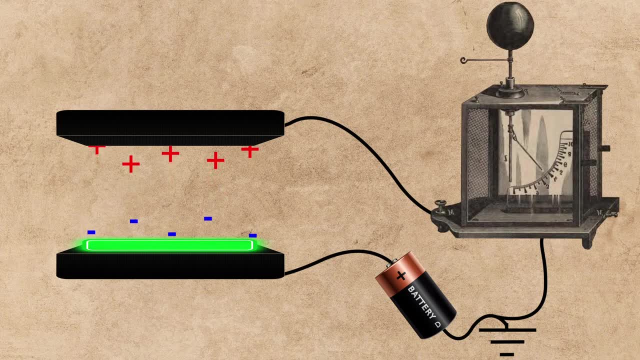 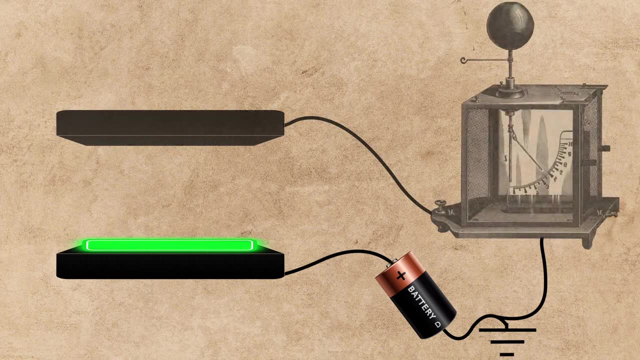 towards the charged plate and the positively charged ions move away from the charged plate. This generates a current in between the plates, which is picked up by the uncharged plate and sensed by the electrometer. The more radiation present, the larger the current measured by the. 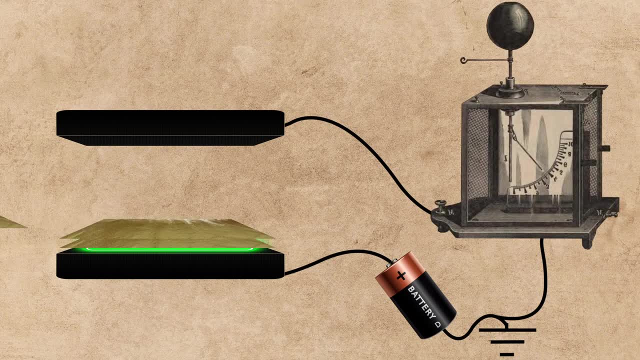 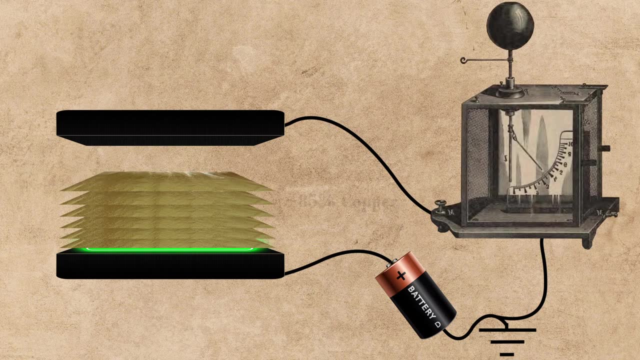 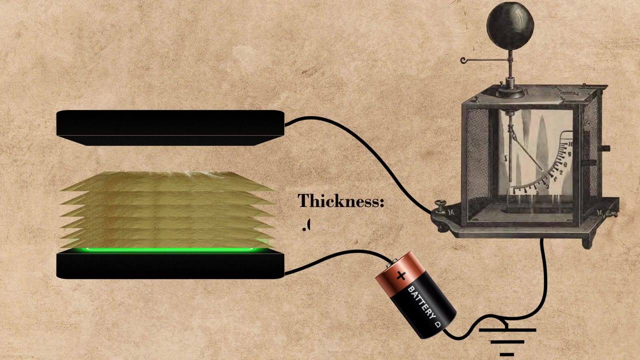 electrometer. For each time he made measurements, he added on top of the uranium a sheet of Dutch metal, which is a form of brass composed of approximately 85% copper and 15% zinc. These sheets were extremely thin, around 0.00008 cm thick, and were added to block some of the 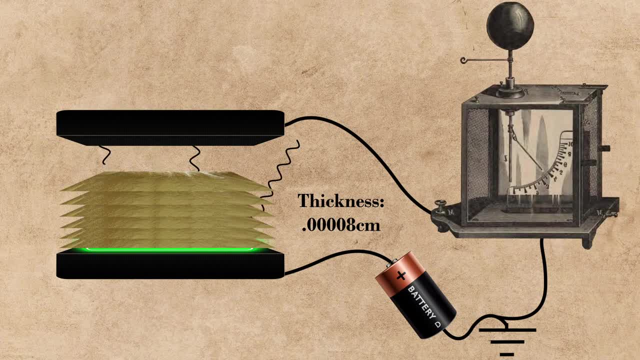 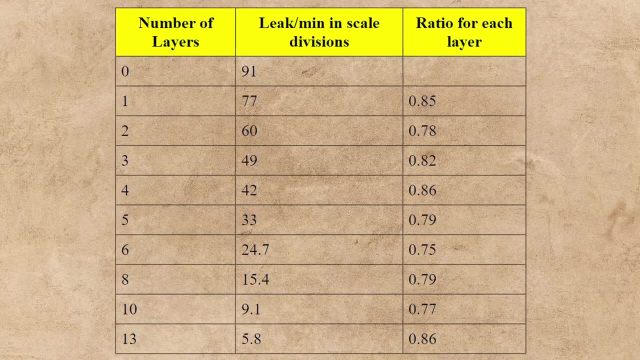 radiation from the uranium into the air between the plates. Rutherford then made measurements of the rate of leak per minute for each sheet of Dutch metal. he added over top the uranium. The results he got from this were somewhat surprising. In this graph you can see how 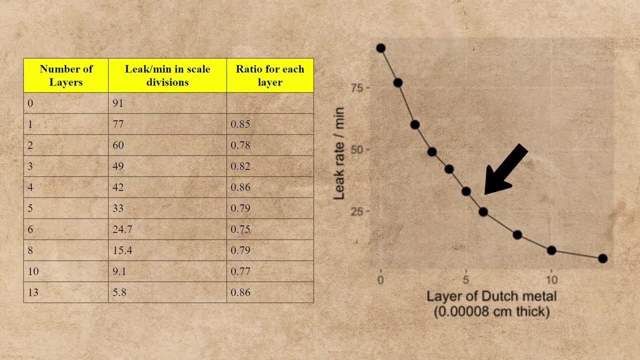 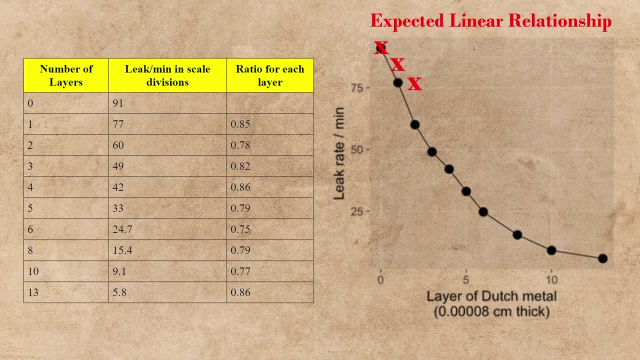 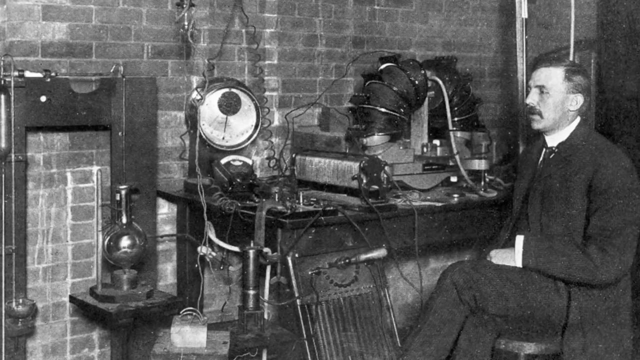 the decrease in radiation is not linear, but rather exponential. If all radiation from the uranium was the same, it would make sense that the radiation would decrease the same amount each time a new layer of Dutch metal was added on top of the uranium. The unexpected results here. 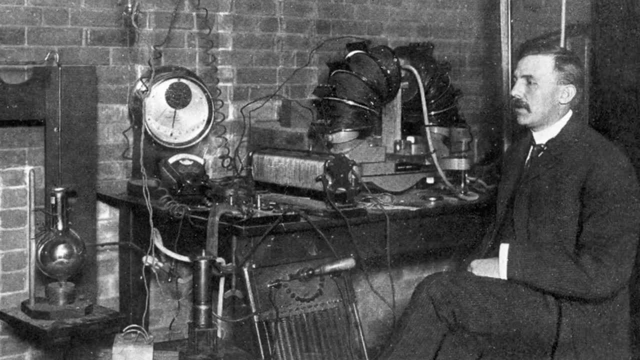 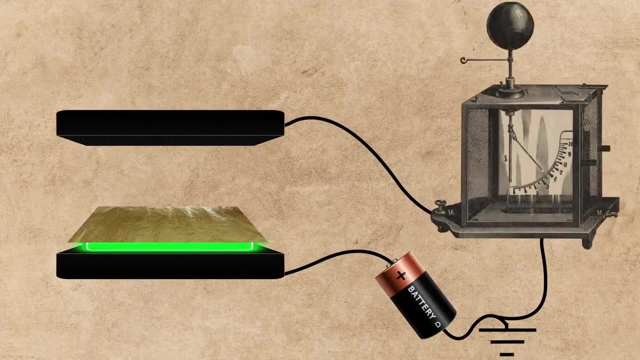 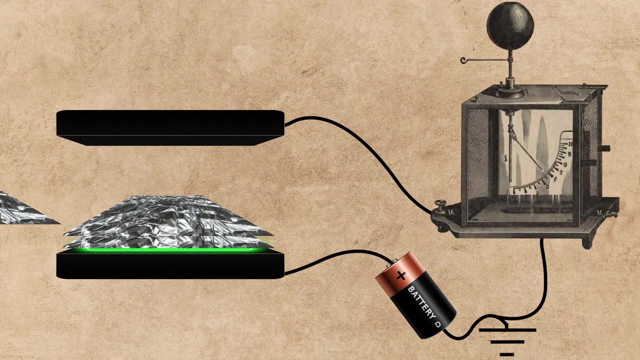 pushed Rutherford to experiment further, this time adding even thicker sheets to possibly uncover a separate layer of radiation. Rutherford switched to 0.0005 cm thick aluminum sheets. This expectedly did a much better job at blocking the radiation, but it only did so for the first few layers added. 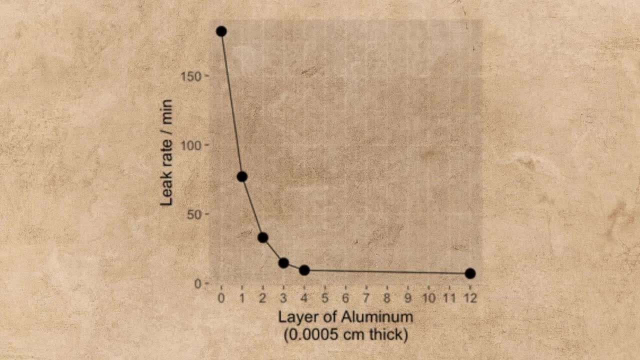 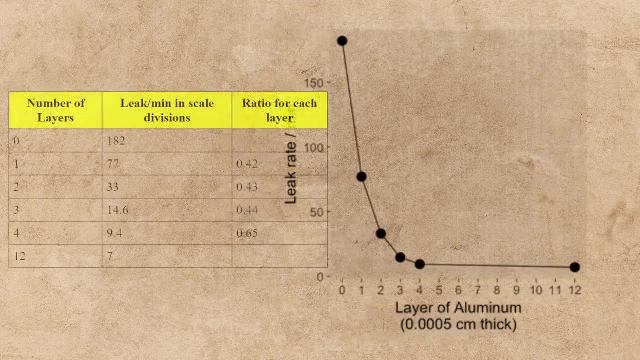 After adding four layers of aluminum foil, the radiation level would remain the same for each new layer of foil he'd added. Rutherford then pushed Rutherford to experiment further, adding over top of the uranium. It would take 12 sheets before Rutherford would see any more. 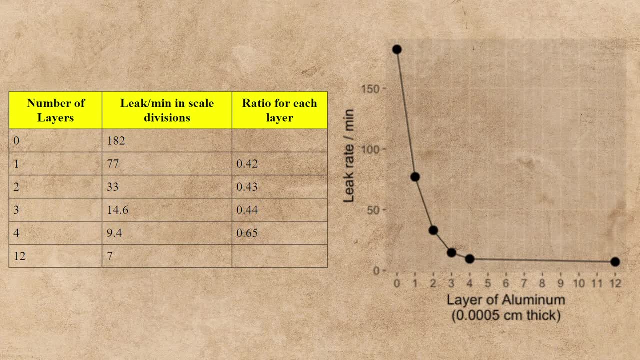 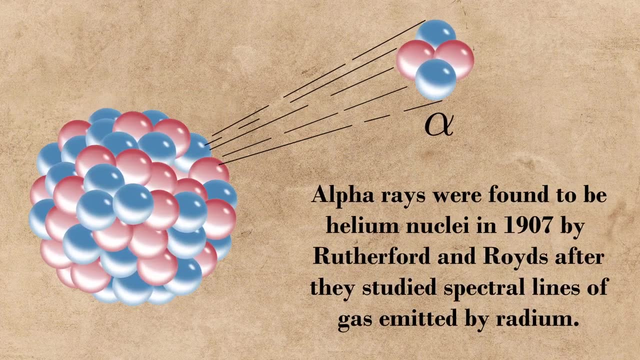 decrease in radiation, which ultimately led him to conclude that there were two different types of radiation from the uranium. The first type, which he called alpha rays, were the easiest to block, and the second type, which he called beta rays, required much more strength to block. 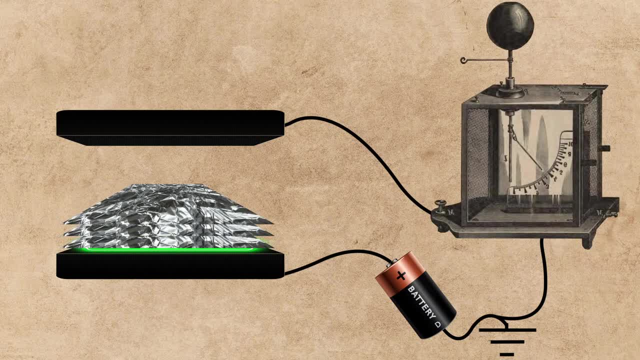 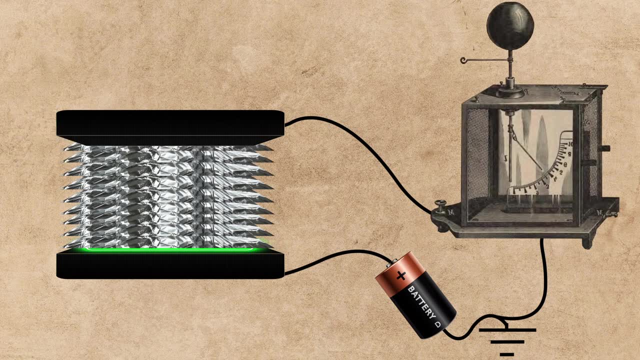 Rutherford then studied beta rays further by continuing to add foil sheets, and he recorded a dataset that showed the difference between the two types of radiation. Rutherford then added a second type, which he called alpha rays, and it required much more strength to block. 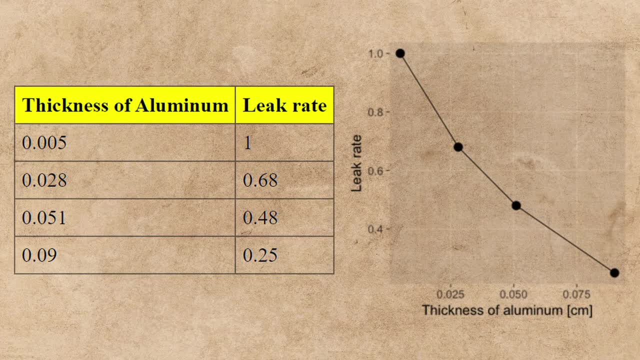 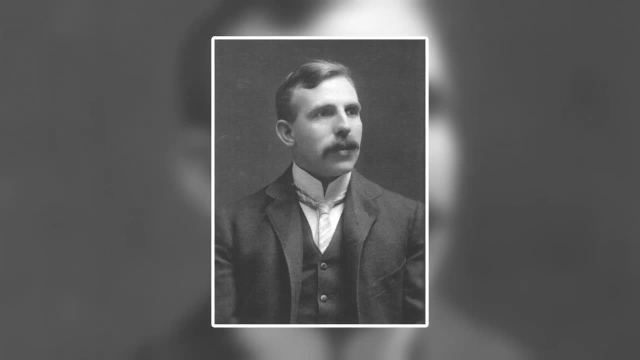 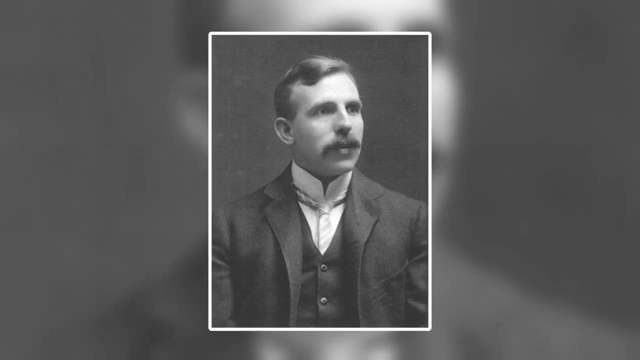 This chart was much more linear than the previous data that contained both types of rays, although not entirely perfect. Rutherford concluded his experiments there, ruling that there was possibly a third type of radiation emitted from the uranium, but that it must have been either so small or so penetrating. 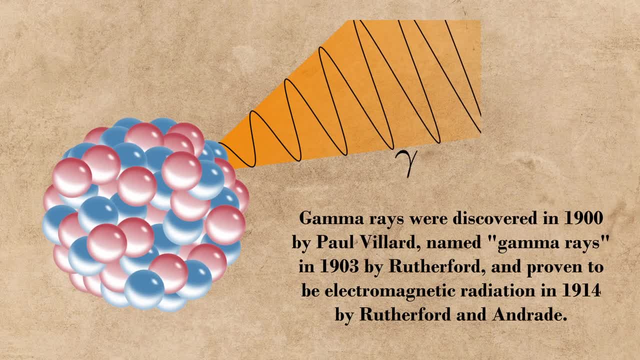 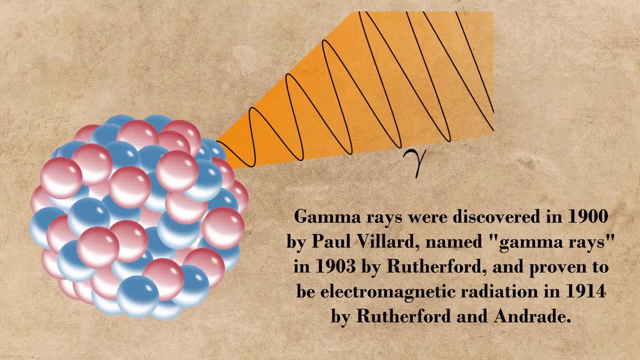 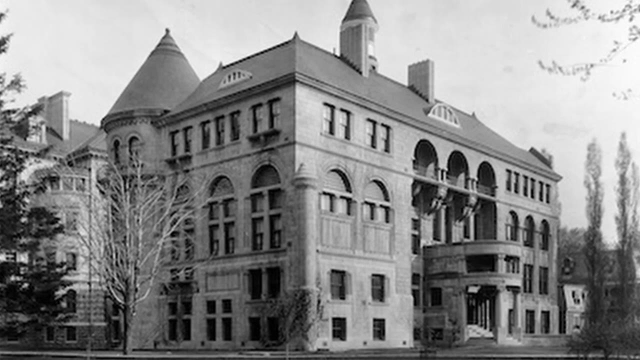 that his experiment could not detect it. This third type would be confirmed a few years later, in 1903, and would be labeled as gamma rays the most penetrating form of radiation. After his discovery of alpha and beta particles, Rutherford moved to McGill University in Montreal. 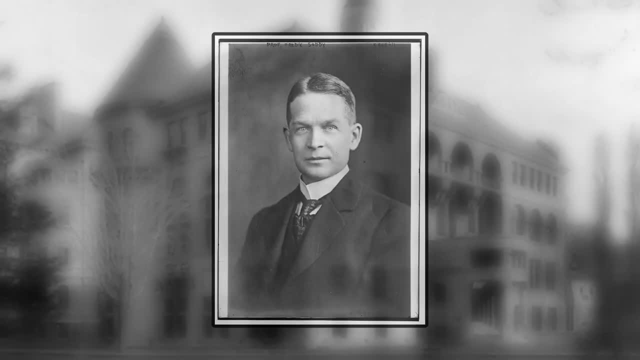 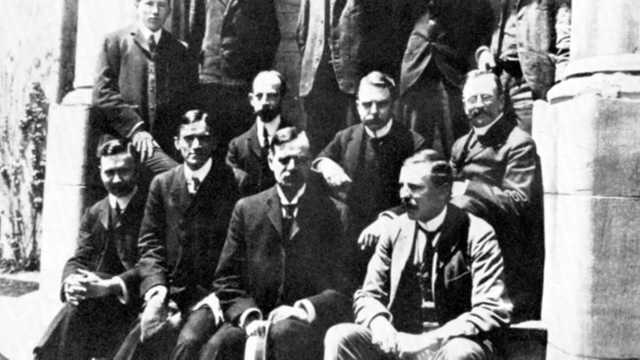 Canada and teamed up with a McGill chemist, Frederick Soddy, to further work on radioactivity During the years of 1902 and 1903, they made another significant breakthrough. Their experiment used a similar setup to that of the one that detected 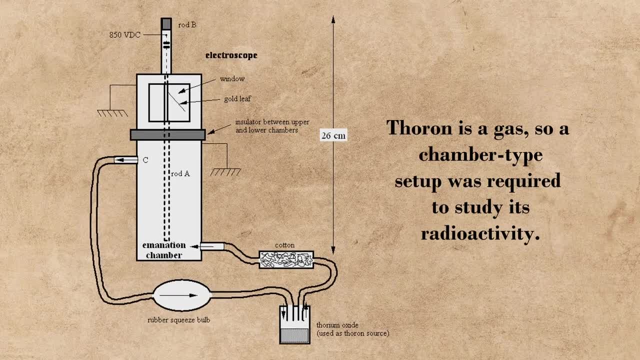 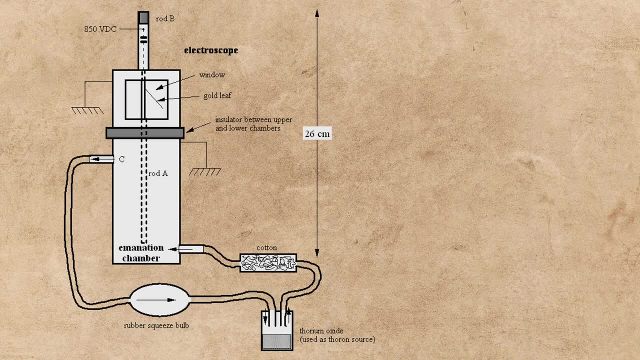 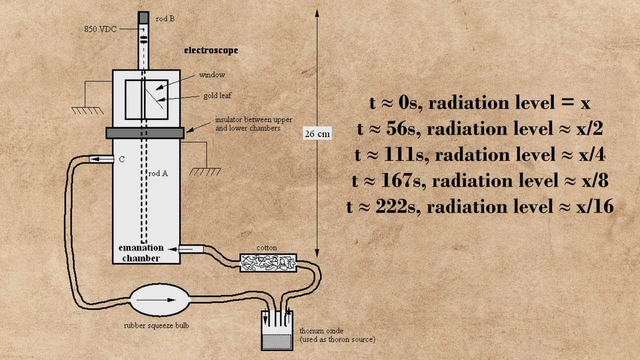 alpha and beta rays, but instead of measuring uranium, it measured an isotope of radon called thoron. While studying thoron, they noticed an interesting trend: that, after identical increments of time, the amount of radiation detected by the thoron at a specific step 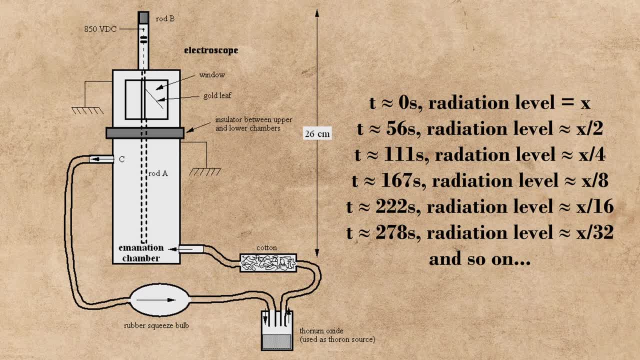 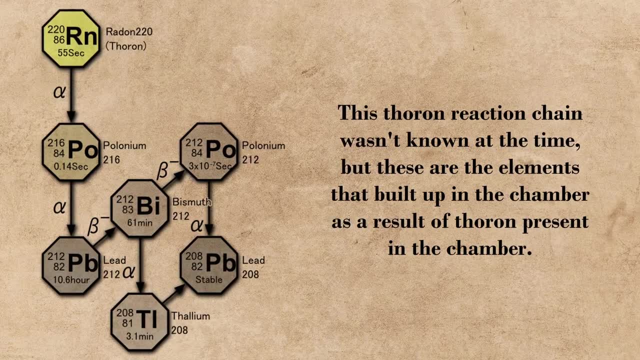 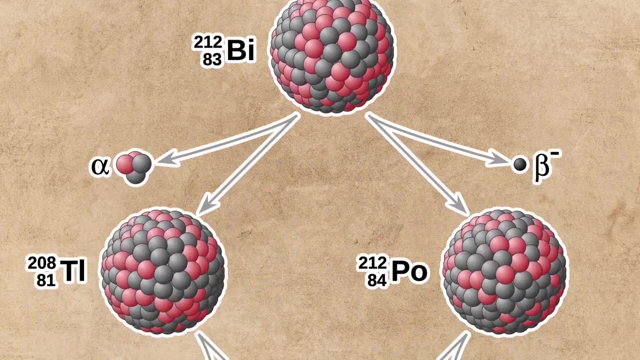 would be half of what it was at the previous step in time. As this was happening, they noticed a seemingly spontaneous buildup of other elements, most notably lead in their setup. From these discoveries, they concluded that over time, radioactive elements must decay. 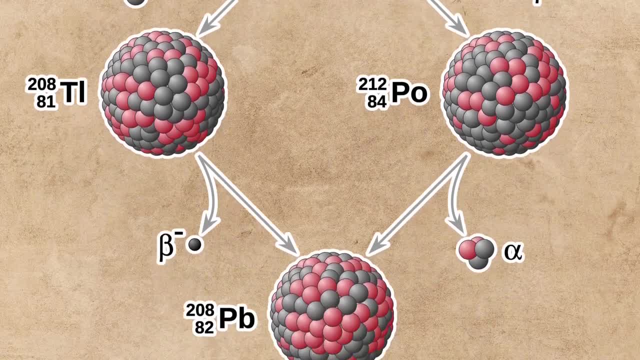 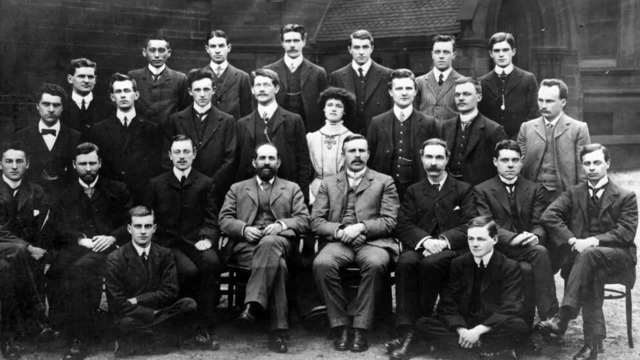 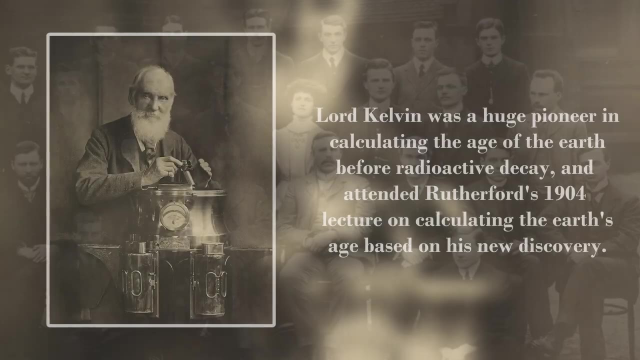 into other elements and introduced the concept of half-lives to the scientific community. Rutherford and Soddy both exploded into scientific fame after these discoveries, sparking debate and controversy over the nature of these results and their implications. Almost immediately after the discovery of radioactive decay, a quest to calculate the true 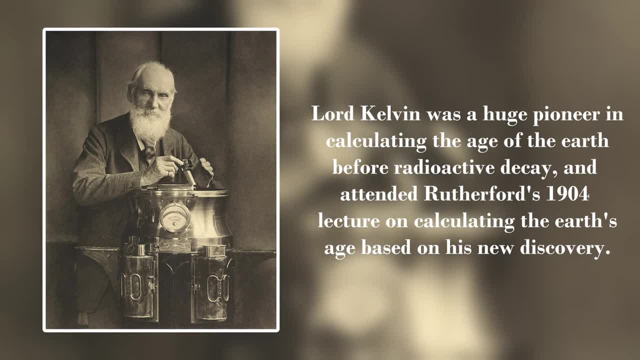 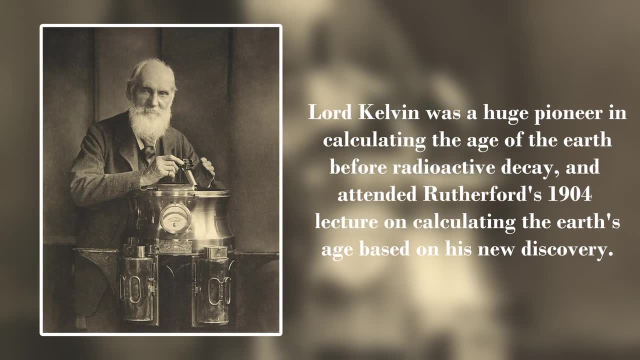 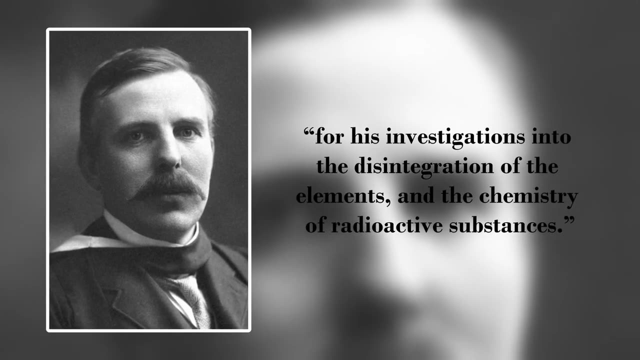 age of the Earth, based on half-lives, was ignited and would make significant leaps in the coming decades. Both Rutherford and Soddy were just getting started too. Rutherford won the Nobel Prize in Chemistry in 1908 for the discovery of alpha particles, beta particles, radioactive decay.